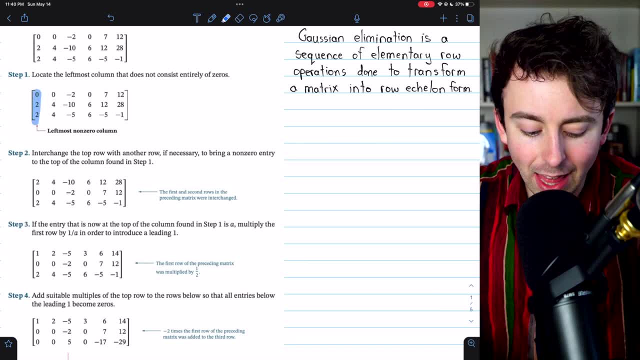 This is where our work begins, And in this matrix the leftmost column does not consist of zeros. So we're going to do two steps here. Step one is to locate the leftmost column of the matrix that does not consist entirely of zeros. 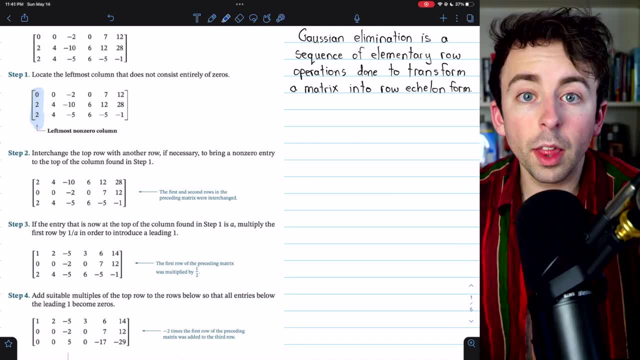 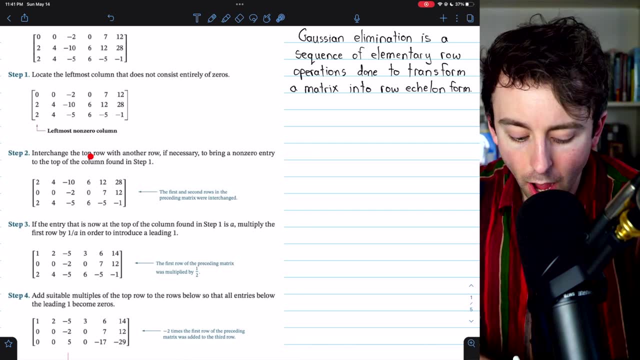 So that's the column we're focusing on. Then we want the top of the column to be non-zero. So step two is to interchange the top row with another row, if necessary, to bring a non-zero entry to the top of the column that we found in step one. 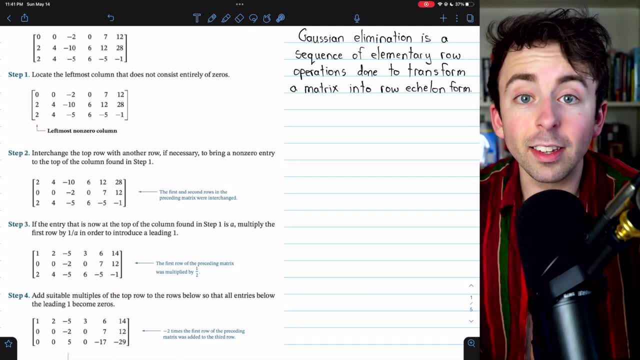 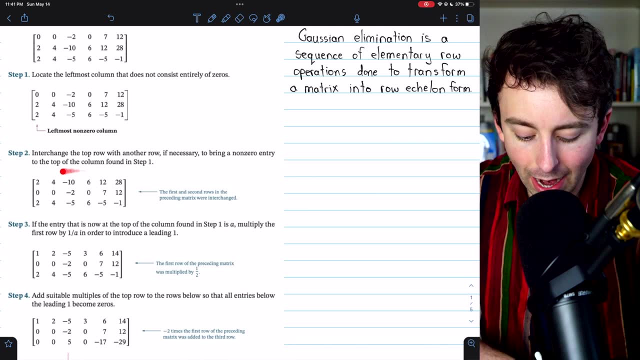 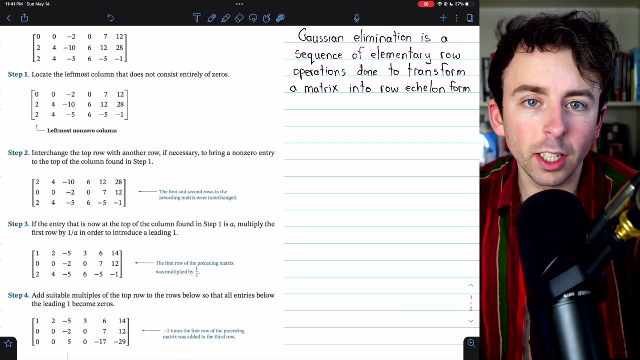 In this case, that entry at the top of our column is zero. So we'll exchange the first row with the second row, And that gets us here After we do step two. So the first and second rows were interchanged And now this first entry at the top of our column is not zero. 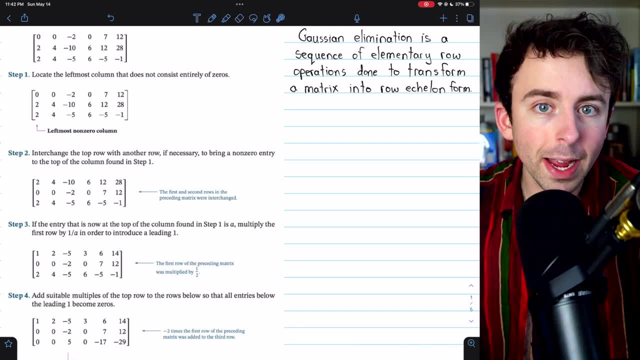 Remember, the goal of Gaussian elimination is to transform a matrix into its row echelon form, which means we want all zero rows at the bottom of the matrix. We want the leading entries to be one and we want zeros below all of those leading entries. 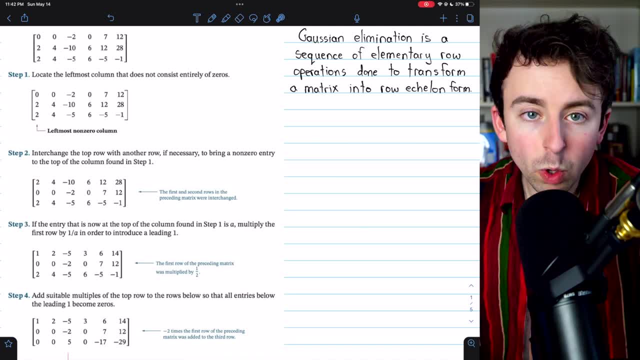 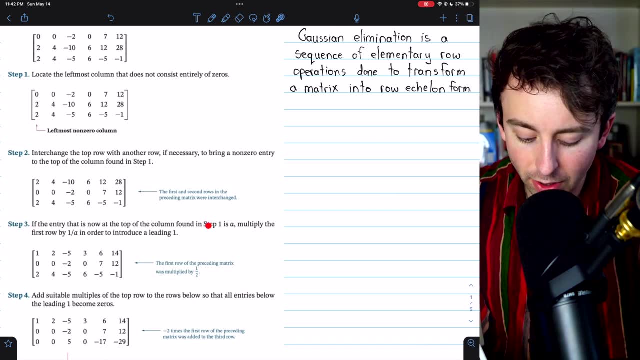 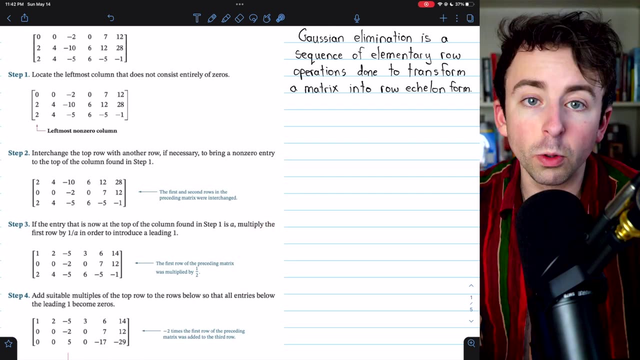 So now that we have this non-zero leading entry, we want it to be one. So step three is, if the entry that's now at the top of the column found in step one is A, we want to multiply the first row by one over A in order to introduce a leading one. 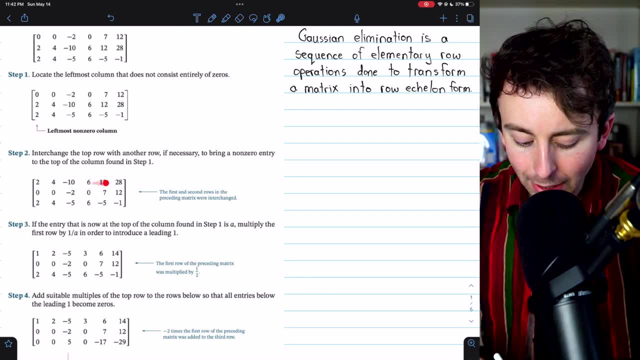 So this entry is two. We want to multiply the row by one over two to turn that two into a one. So we multiply by a half. The two becomes a one, as desired. The four becomes a two. Negative ten becomes negative five. 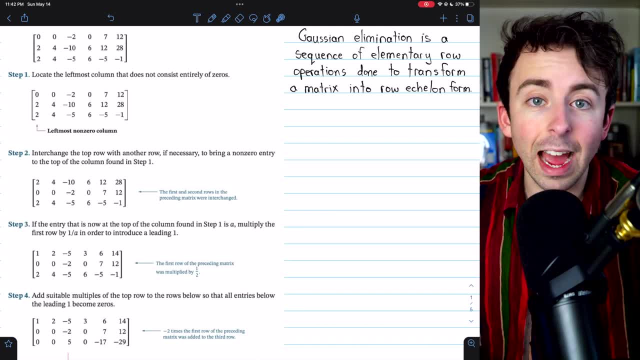 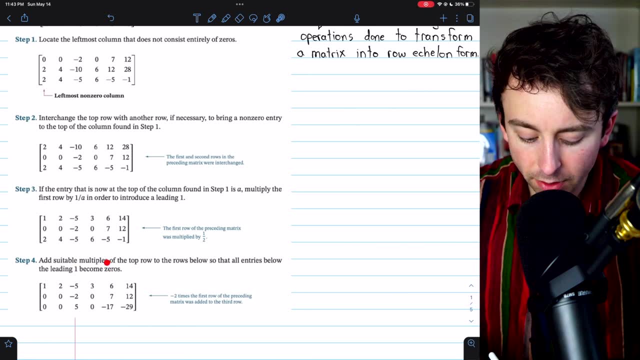 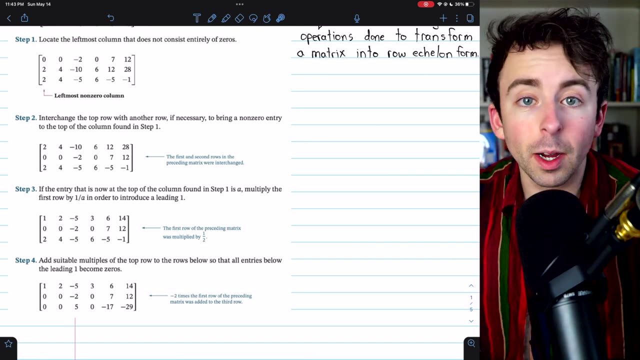 And so on. But, importantly, this leading entry is now a one And the use of having a one as the leading entry is. now it's easy to add suitable multiples of this top row to the rows below so that all the entries below the leading one become zeros. 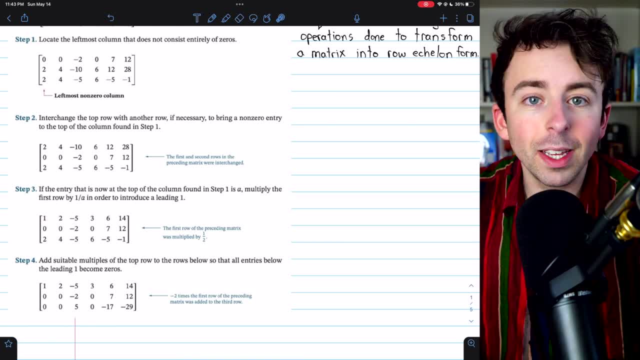 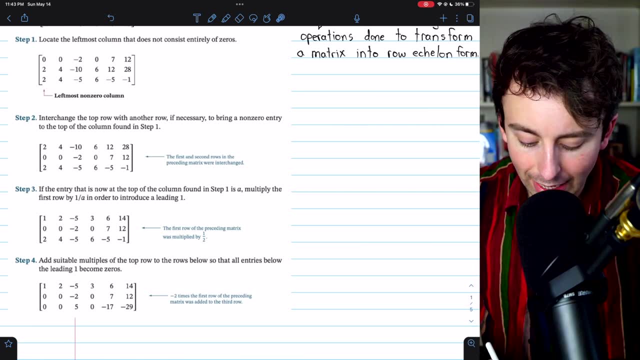 We've got this two below the leading one. We want that to be a zero, So we just add negative two times row one to row three. So negative two times the first row gets added to the third row. And now we have this matrix. 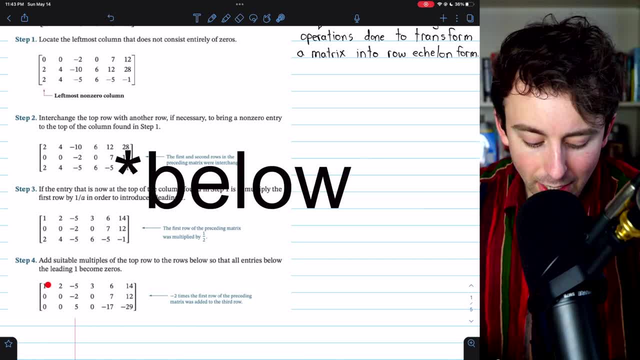 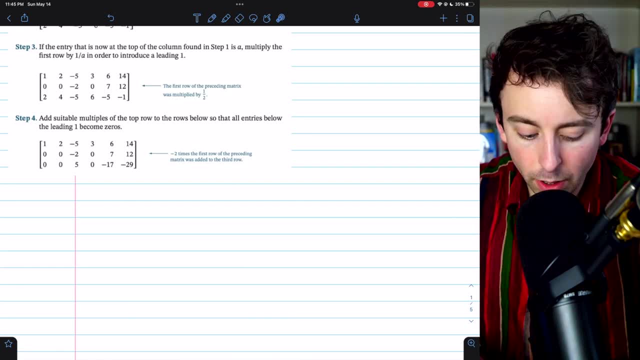 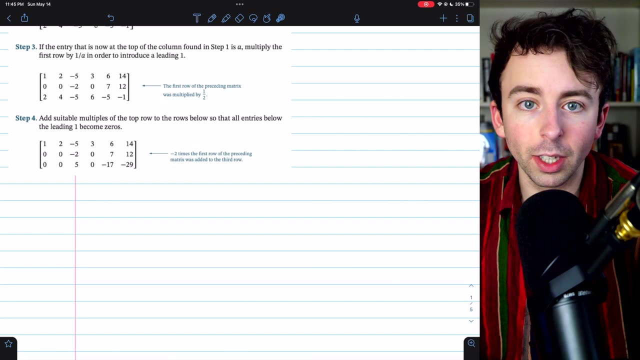 And, importantly, we see there are all zeros between the one in this first column. With the goal of getting this matrix into row echelon form. our work with row one and column one is now done. We have a leading one in the row and the column has zeros below the leading one. 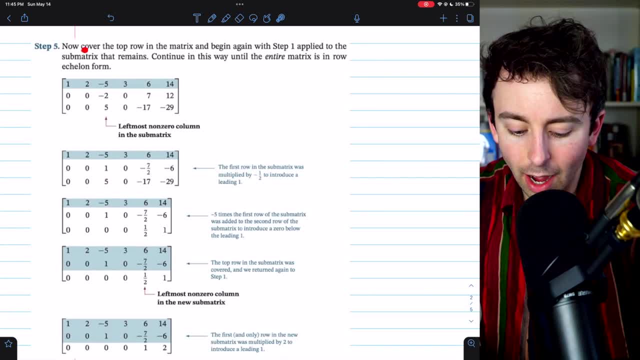 So we can move on to step five, where we essentially cover the top row in the matrix and begin again with step one, But now applied to the sub matrix that remains once we cover up row one. So in this sub matrix we again identify the left most non zero column and continue. 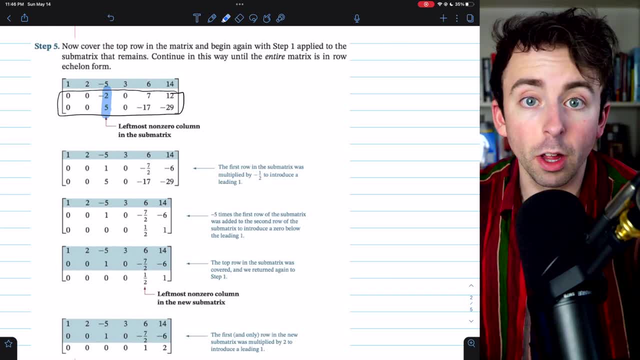 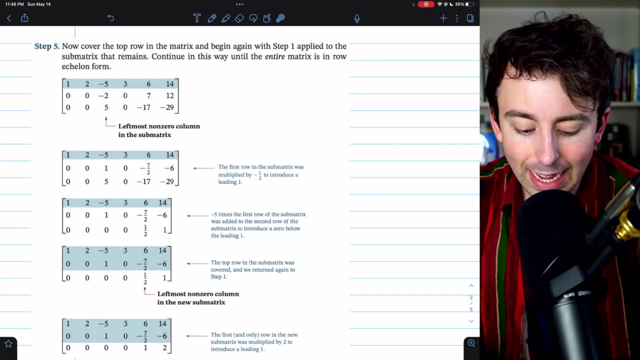 repeating the steps as before until the matrix is in row echelon form. So here in this left most column, our leading entry, ignoring row one, because our work with that is done is negative two. We want that to become a one. 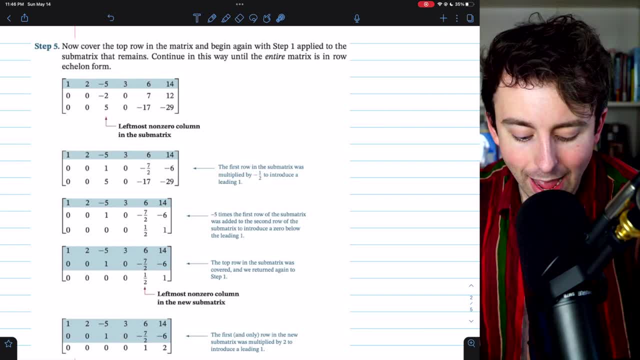 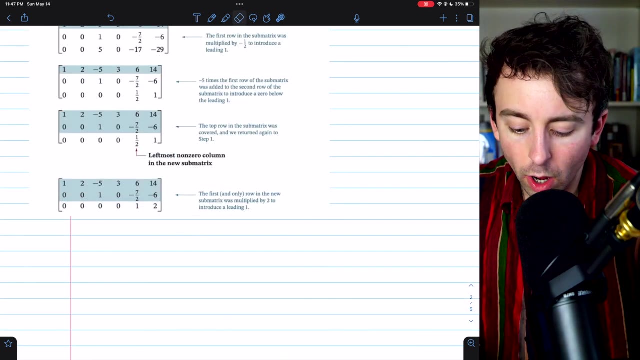 So we multiply row two by negative one half, And then we can use this one and add negative five copies of row two to row three. That way we turn this five into a zero and proceed in this manner. Once we get this leading entry to be a one, our work with row two is done. 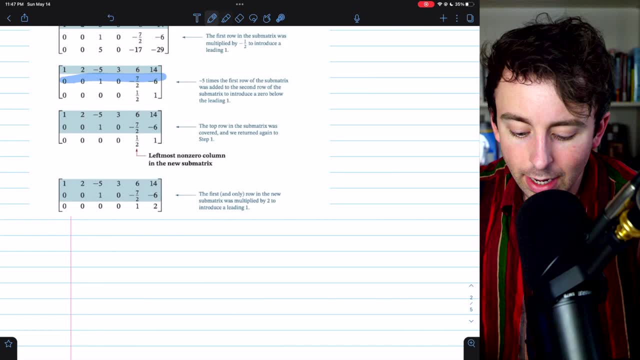 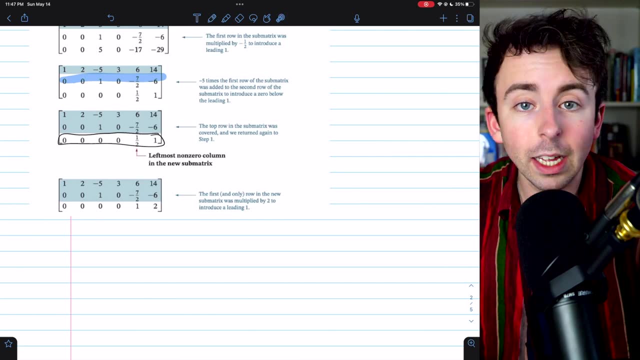 So we can cover up the row and go back to step one, Now, focusing on the very small sub matrix that remains. The only step left is to multiply row three by two in order to turn its leading entry into a one, And this matrix is now in row echelon form. 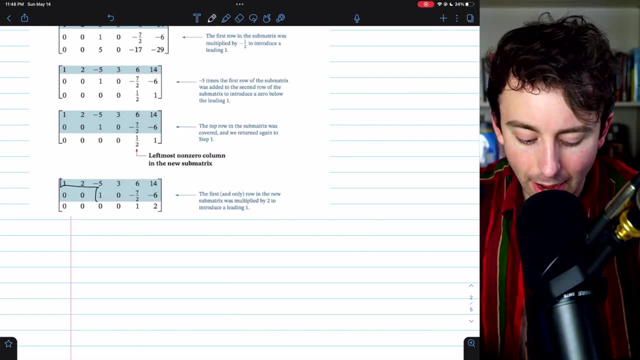 The leading entries are all ones that have this staircase pattern where each leading one is further to the right than the leading one above it. Any row of all zeros is at the bottom of the matrix. In this case, there is no row of all zeros and each leading one has zeros below it. 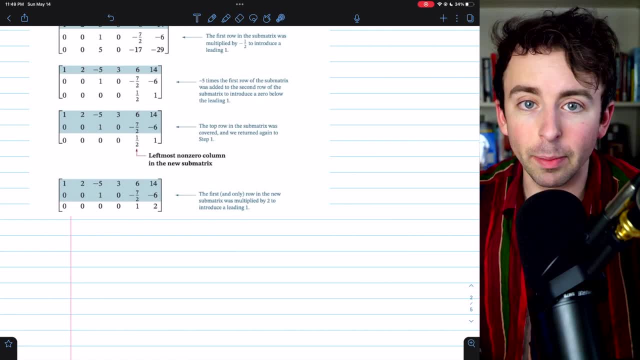 So this is in row echelon form. We have completed Gaussian elimination. now that the matrix is in row echelon form, We can solve the system of linear equations that it might represent. to use Gaussian elimination in order to solve a system of linear equations: 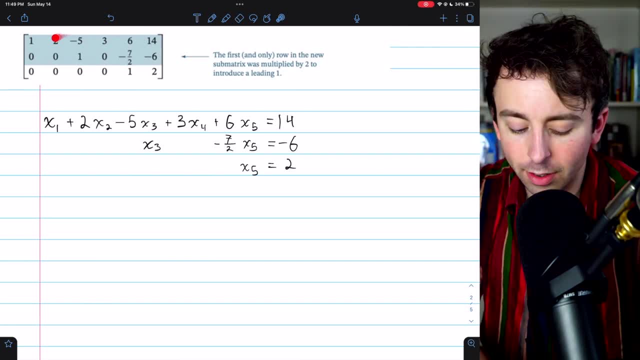 Once you complete the Gaussian elimination and get the matrix into row echelon form, you can take the matrix and turn it back into a system of linear equations. that gives us this. we're just taking the coefficients, So one X one plus two X two minus five. 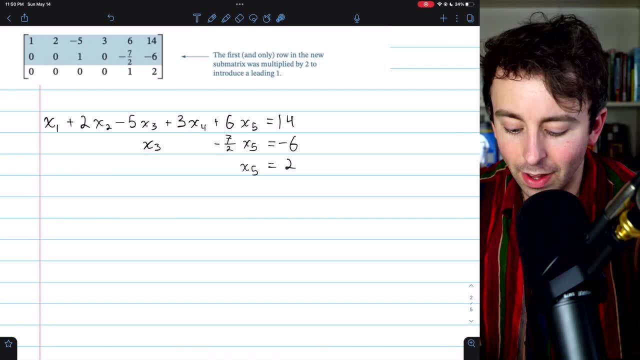 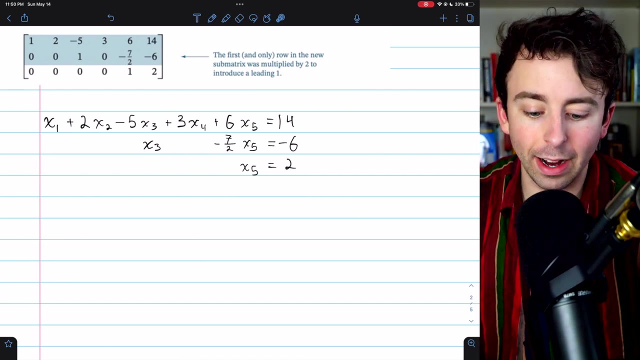 X three plus three, X four plus six X five equals 14, and so on. for the other rows, Notice, in the equation from row two, for example, I haven't written zero X four. I have just included this space here, though, so you can see there are no X fours in this second equation. 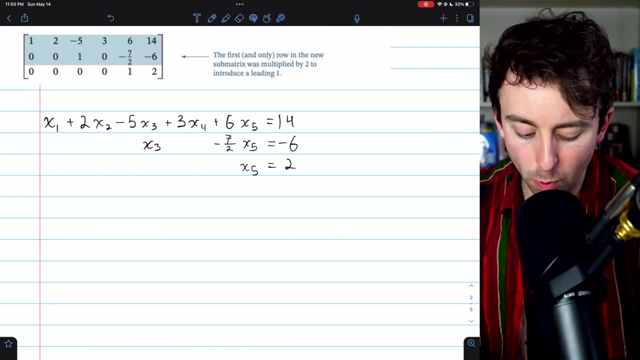 Once you have your reduced system of equations that comes from that row reduced echelon form, you want to solve for the leading variables. So everything except the leading variables, except X one, we move to the other side of the equation. So X one equals 14 minus two, X two, and so on. X three: 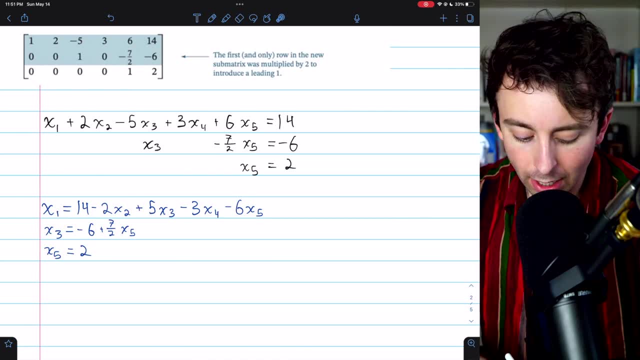 We added seven halves X five to the other side of the equation. So X three equals negative six plus seven halves X five, and X five is just equal to two. So again you get your system of equations and then solve for the leading variables. 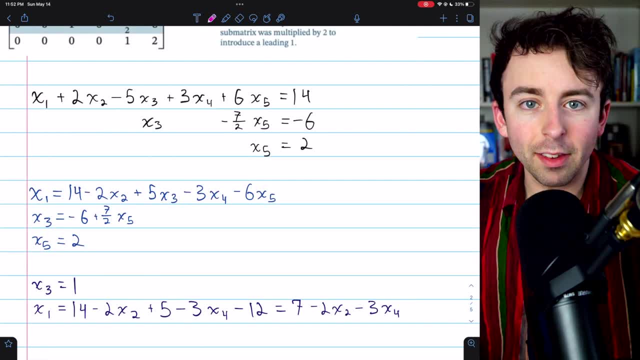 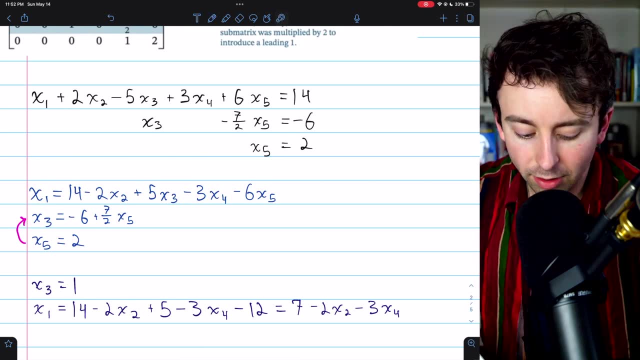 Those are the variables in the front. Then we complete a simple process called back substitution, Beginning with your bottom equation. plug it in to the above equation. So X three is equal to negative six plus seven halves X five. But we know X five is equal to two. 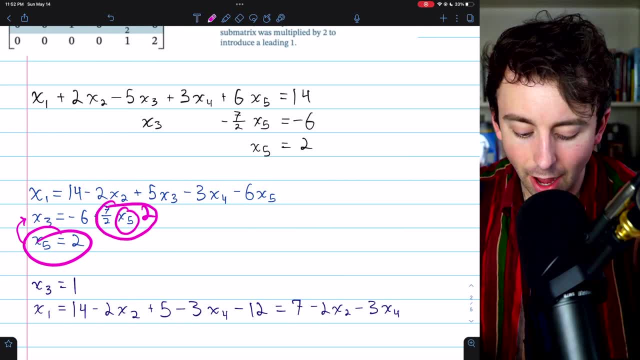 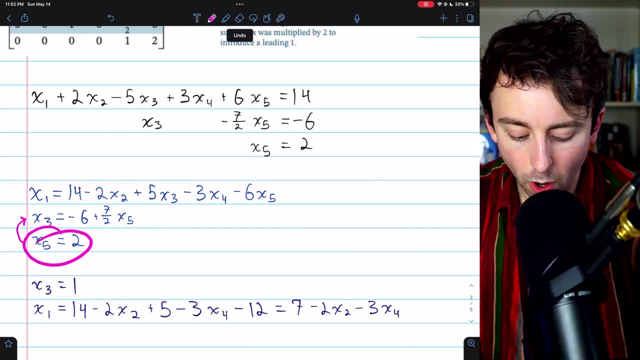 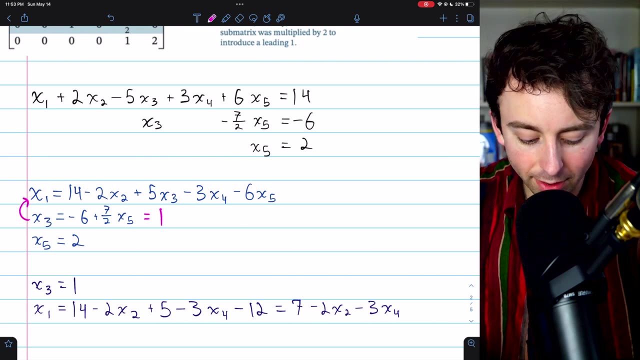 So if we plug two in here, we have seven halves times two, which is just seven, and negative. six plus seven is positive one, And so we have the X. three is equal to positive one. Then we plug these two equations into the above equation. 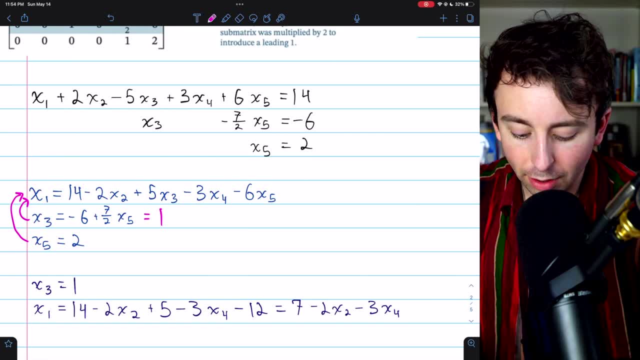 X one is equal to 14 minus two X two, plus five X three, But we know X three is equal to one. So this is just five minus three X four, and then minus six X five, But we know X five is equal to two. 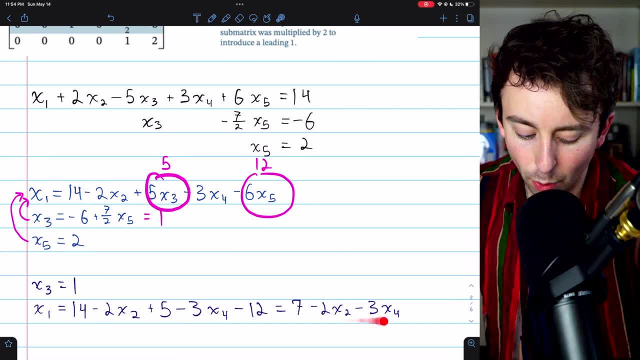 So six X five is just twelve, And that gives us this equation: X one is equal to 14 minus two X two plus five minus three X four minus twelve. Combining the 14, the five and the minus twelve, we have the X one equals seven minus two X two. 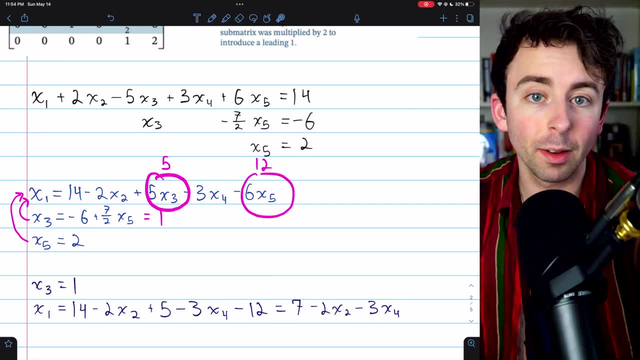 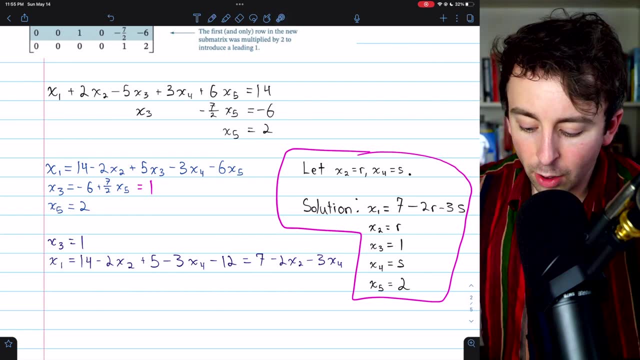 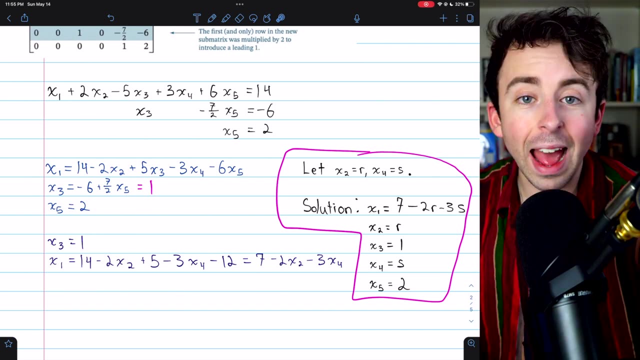 minus three X four, and we've completed this back substitution process And with that we can describe the general solution. with these parametric equations We see that X two and X four were free variables right X two, X four. They don't have any restrictions in our system of equations. 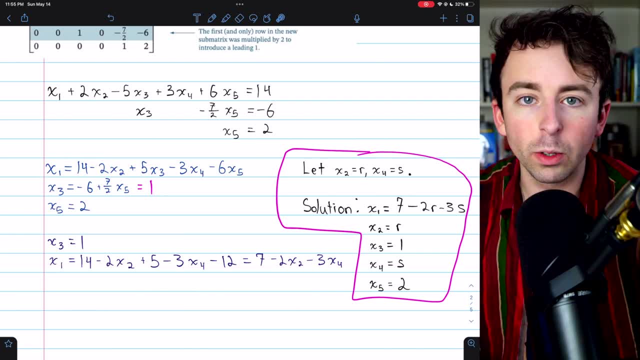 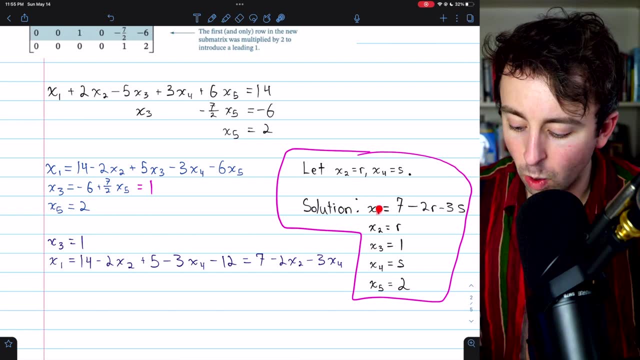 So we'll just say: let X two equal R and X four equal S. Those are just parameters. We're calling them R and S. So then our solution is this set of equations: X one is equal to seven minus two X two. 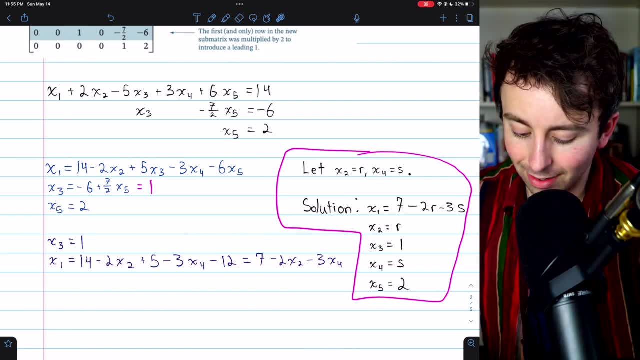 But X two is R. So seven minus two, R minus three times S. X two is a free variable. It's equal to R. X three is equal to one. We figured that out. X four is a free variable. It's equal to S and X five. 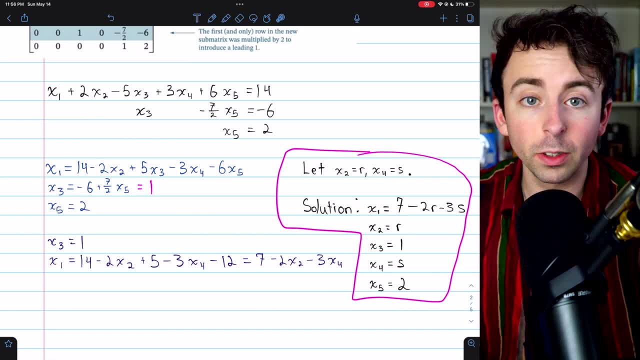 We figured out It was two, And this is the general solution. So if you represent a system of linear equations as a matrix, this is how you can use Gaussian elimination in order to solve it. You're not always going to need parameters to describe your solutions. 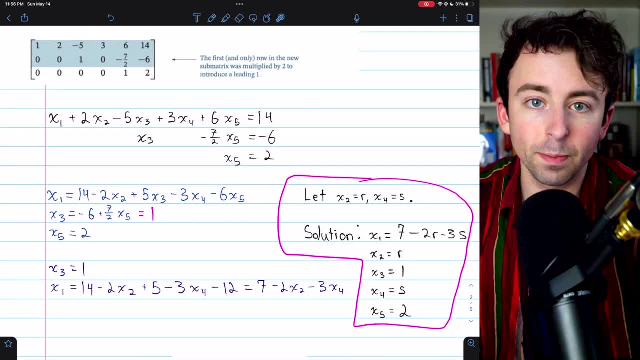 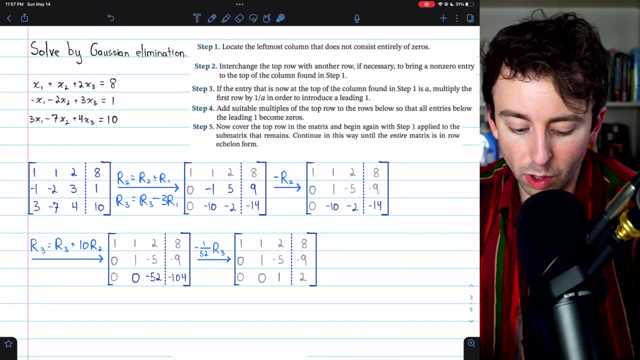 We did in this case, though, because we have more unknowns than we have equations, So there's going to be some free variables. In this example. there will not be parameters in our solution. We've got three equations and we've got three variables. 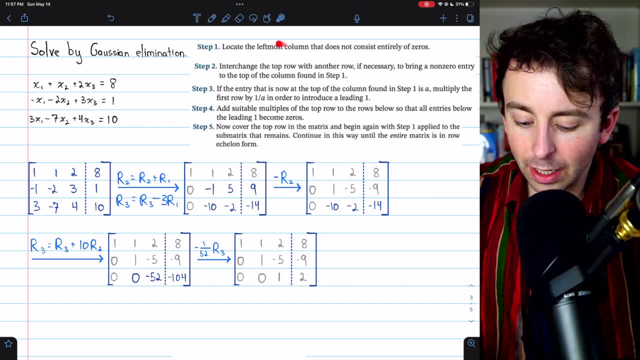 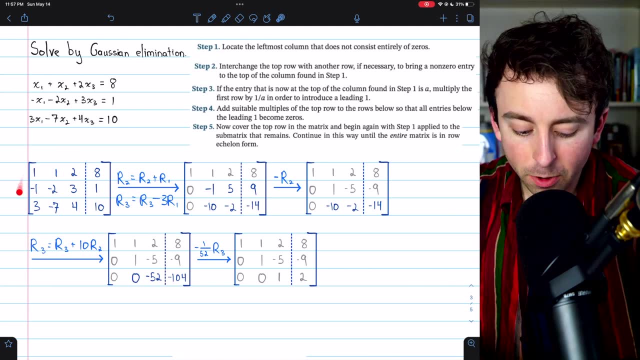 Let's solve this system- Gaussian elimination- And I've included the five steps here for your reference. The first thing we do is take our system of linear equations and represent it as an augmented matrix. So the coefficients of the X ones are in column one. 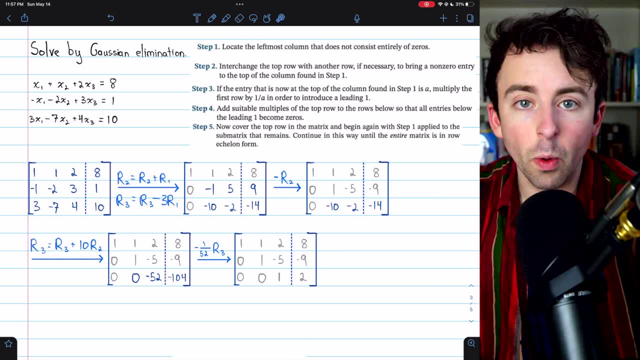 The coefficients of the X twos are in column two and so on, with the constants in column four, which, just to make it easier to look at, I've separated with a dotted line, though that is not necessary. We begin by identifying our left. 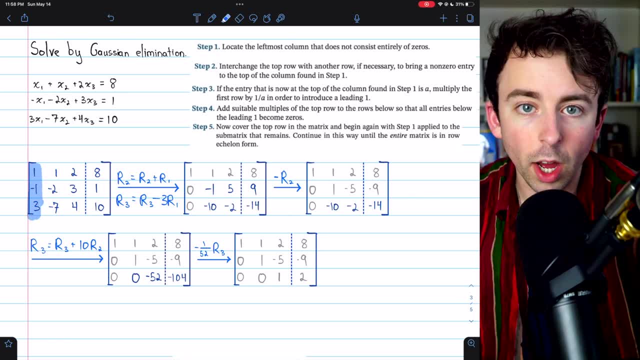 Most non zero column- in this case it's column one. Then we want to turn the entry at the top of column one into a one. In this case it's already a one. So we are already on to step four, where we need to add suitable multiples. 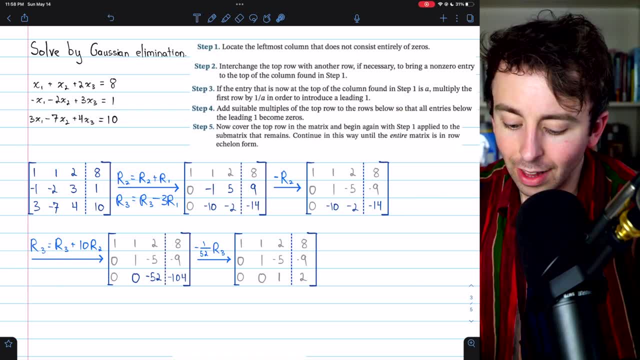 of the top row to the rows below, so that all entries below the leading one become zeros. So to do that, we'll add one copy of row one to row two, turning that negative one into a zero. And we'll Add negative three copies of row one to row three, turning this three into a zero. 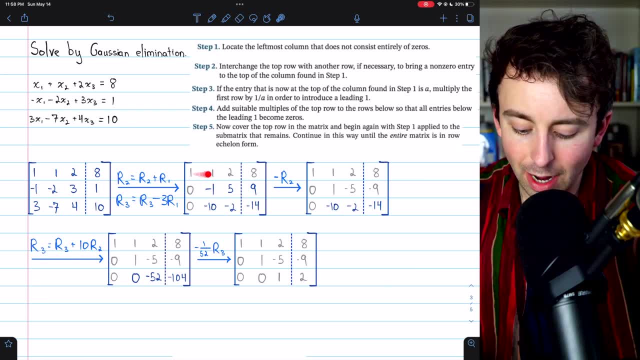 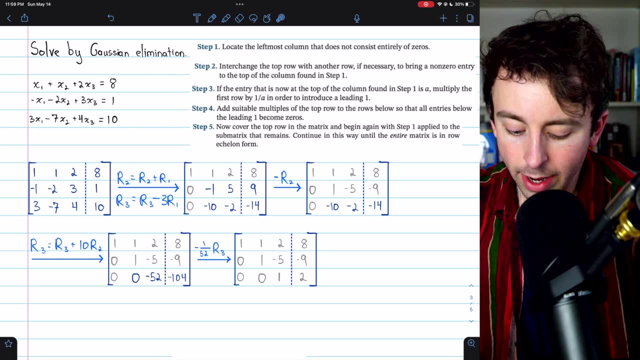 This is the resulting matrix, And I've put some of these numbers, namely column one and row one, in gray because our work with them is now done. We have this leading one and zeros below it, So we now repeat the process focusing on this sub matrix. 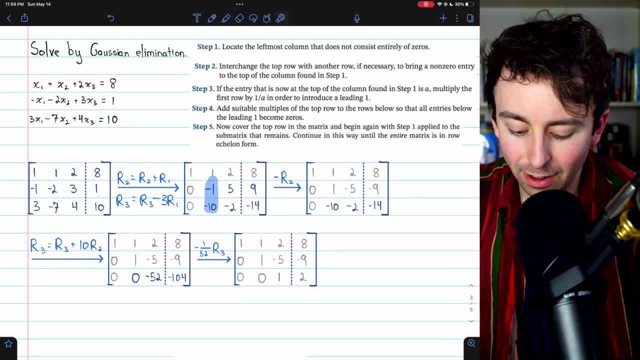 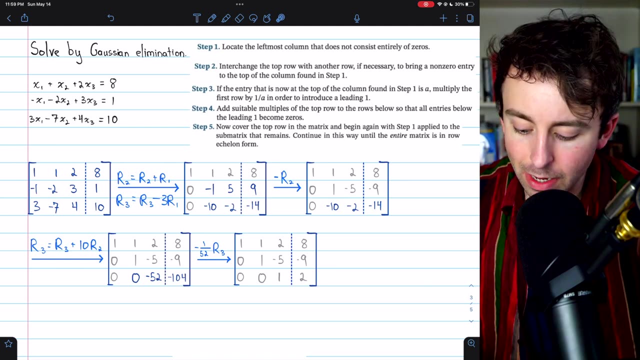 The leftmost column is column two, and the leading entry here at the top is negative one, So we'll multiply row two by negative one in order to turn that leading entry into a positive one. Now our work with this row is done, but we still need to add ten copies of row two. 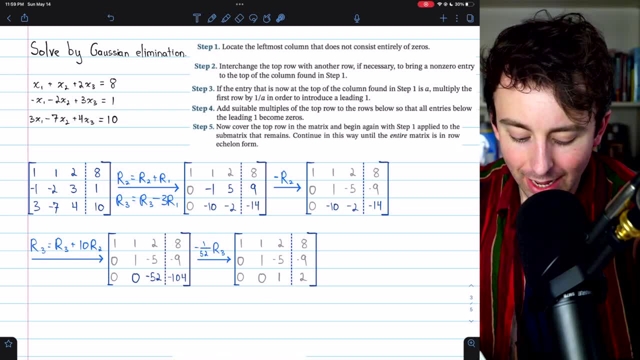 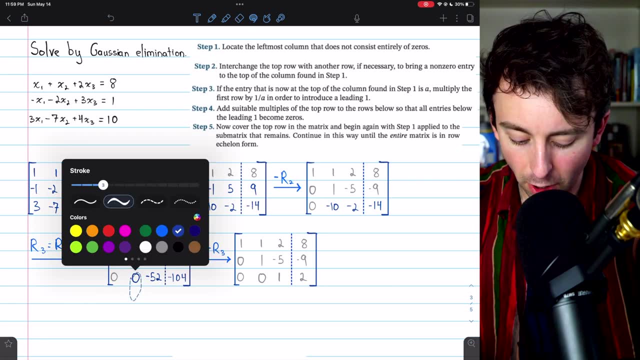 to row three in order to turn this negative ten into a zero. And that gets us here. to be consistent in my coloring, I should turn this zero into a gray, because our work with this column is now done And we're focusing on this. 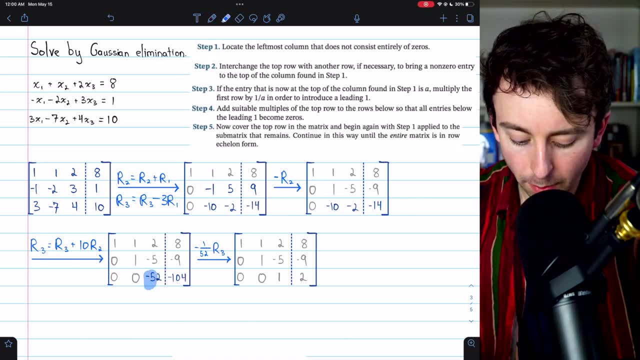 Sub matrix. now our leftmost non zero column is column three, And the only step that remains here is to multiply row three by negative one over fifty two to turn this leading entry into a positive one. And now we've got the matrix in row echelon form. 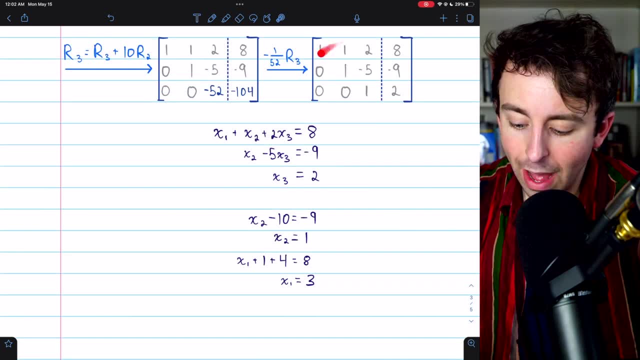 We've completed Gaussian elimination. Then we take our row echelon matrix and turn it back into a system of linear equations. That gives us X one plus X two plus two, X three equals Eight, X two minus five, X three equals negative nine and X three equals two. 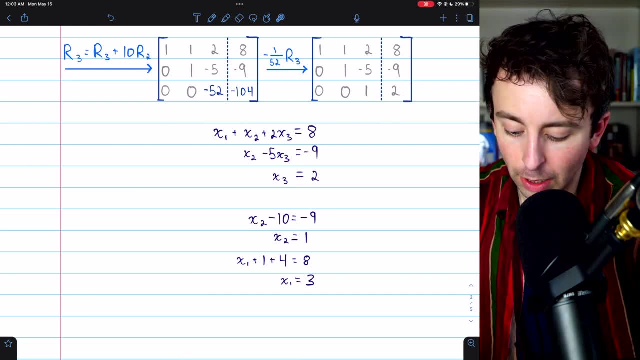 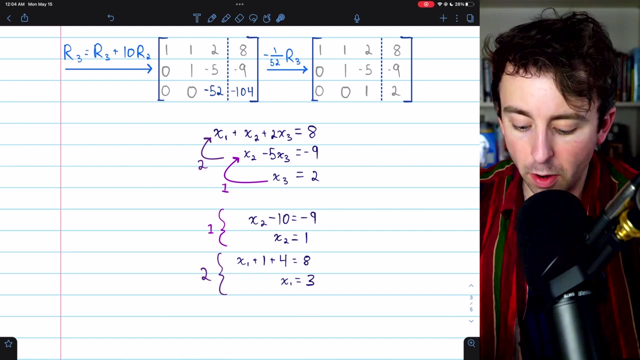 We then carry out that back substitution process, plugging this into this and then this into this. First we plug X three equals two into this equation. giving X two minus ten equals negative nine, And so X two is equal to one. Then we can plug all of our known information into this equation. 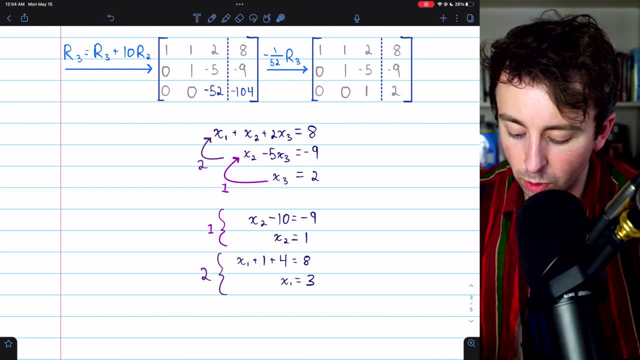 So we have X one plus X two, which is one. So X one plus one plus two, X three, X three is two. So that's plus four equals eight, which means X one equals three, And so we have the solution to the system. 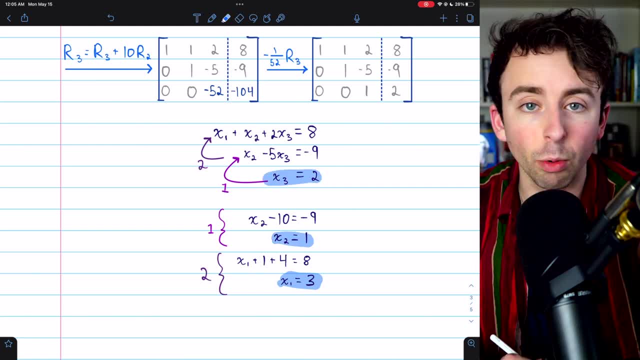 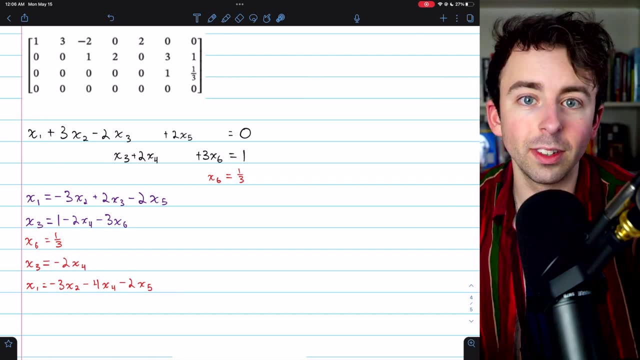 X one equals three, X two equals one and X three equals two. Here's one more example, if it's useful, where again we have free variables. We've got more unknowns than equations. So this is a matrix, having already had Gaussian elimination done to it. 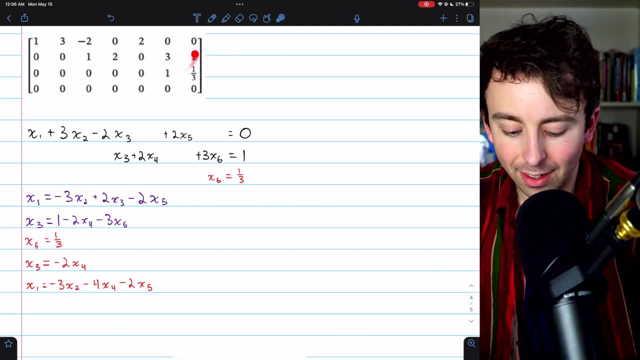 It is in row echelon form, So we can take this and turn it into a system of equations, which we see here. These three equations- I've made this one red because it's already a final solution- The other two equations we need to solve for the leading variables, since they're 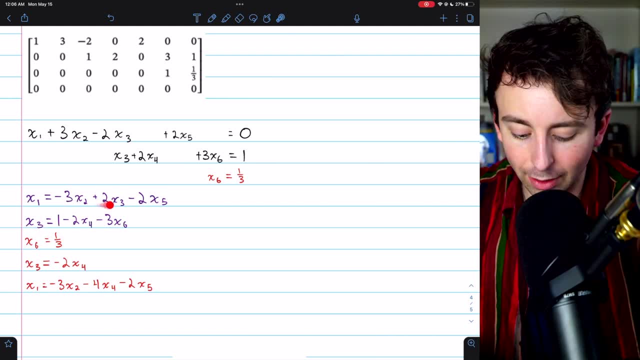 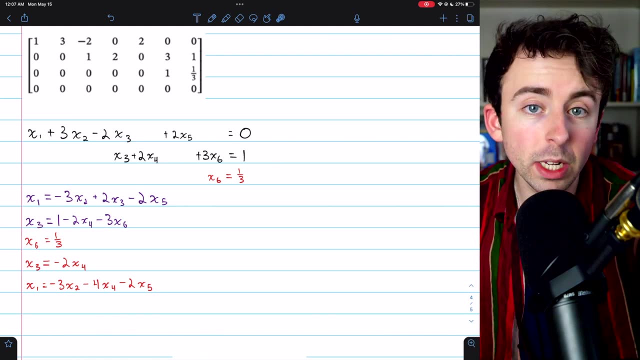 not already solved for the leading variable that gives us this: X one equals move all this stuff to the right, and X three equals move all of this stuff to the right. And then we do that back substitution process. We know already that X six is equal to one third. 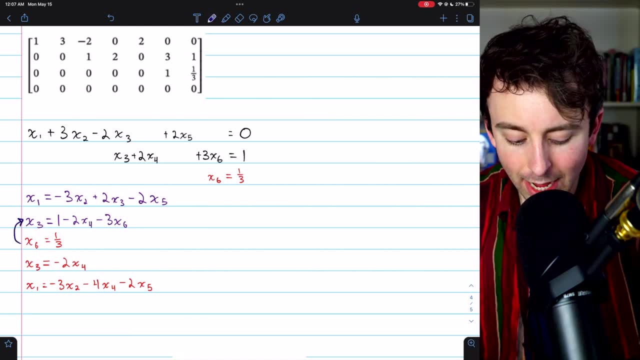 So we can take that and plug it in to X three. That gives us the X three is equal to one minus two X four minus three times a third, which is just minus one, And that minus one cancels out with that plus one, which leaves X three equals negative two X four. 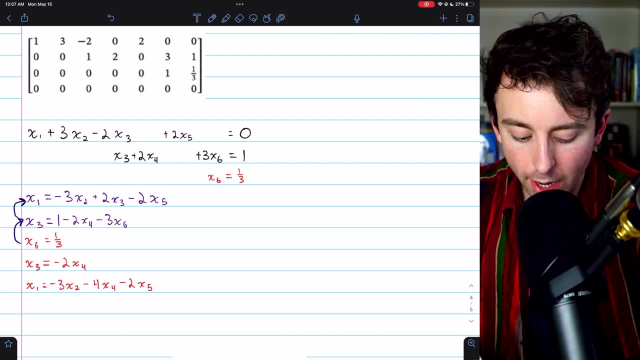 That then gets plugged in to our equation, for X one X one equals negative three X two plus two X three. But we know that X three is minus two X four, So that's just minus four X four and then minus two X five. 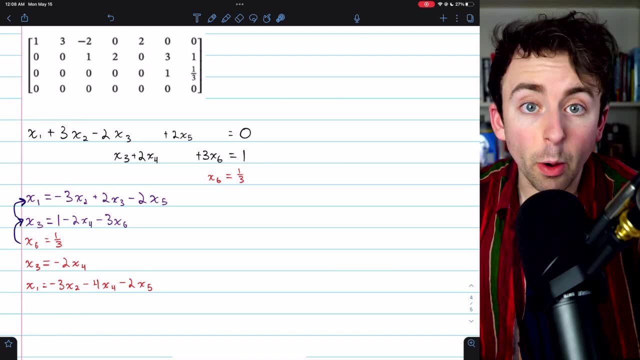 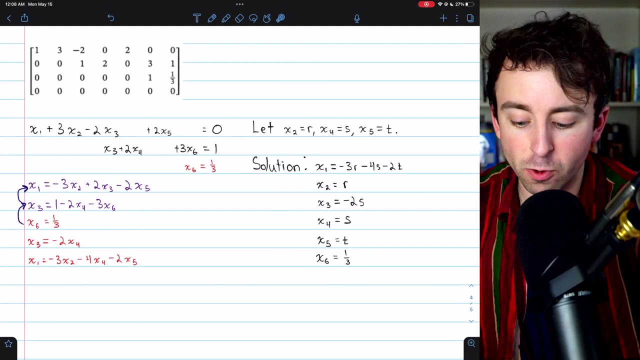 And that's our equation for X one. So you can see, our free variables are X two, X four and X five. They can be whatever they want, whereas there are restrictions on X six, X three and X one. And so here is the general solution in terms of parametric. 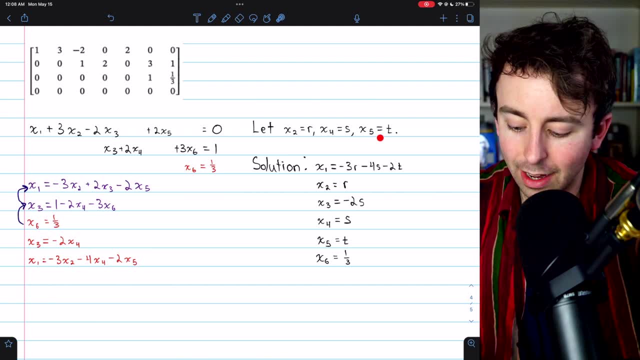 Equations: X two is our X, four is S and X five is T. Again, these are free variables, so we'll make those. our parameters are S and T. The solution then is: X one equals negative three, R minus four, S minus two, T, X two equals R, X three. 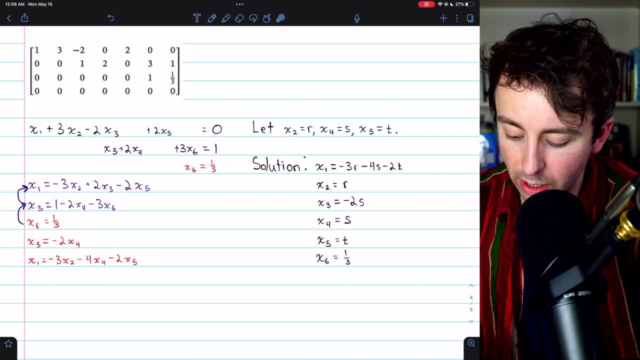 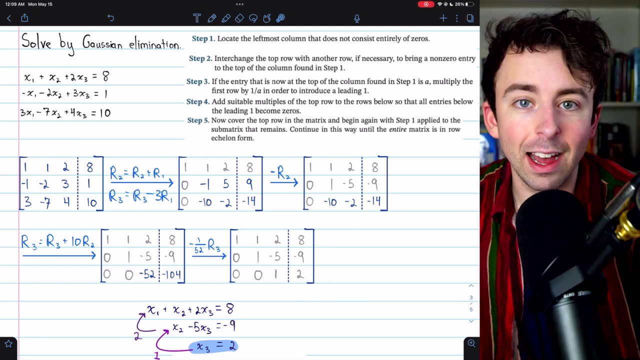 equals negative. two S X. four equals S X. five equals T and X. six, of course, is one third. And here are the steps again. in case you want to have another, look. that's your guide to Gaussian elimination. Again, you don't have to follow these steps. 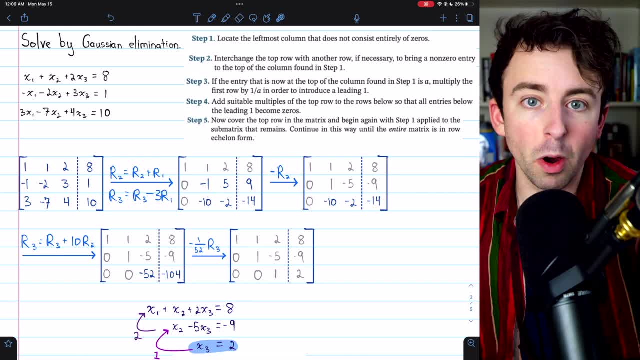 If you know the goal of Gaussian elimination, just perform whatever row operations you feel like, but you might find it more efficient to follow the same procedure each time. That's how you do it And that's how you can use it to solve a system of linear equations.